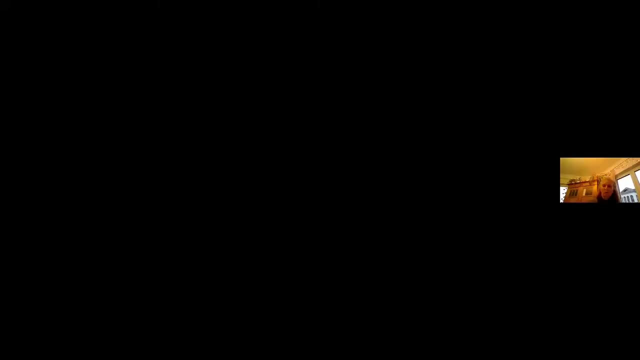 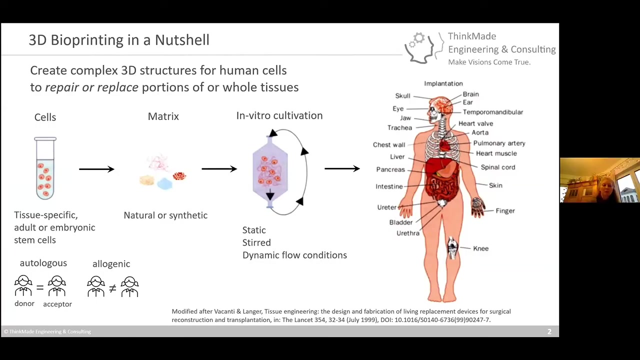 This kind of works about almost 20 years ago and not really coming from the biology part but from the optics and photonics part. So 3D bioprinting- we heard it a lot today- is the idea to create complex 3D structures for human cells to repair or replace. 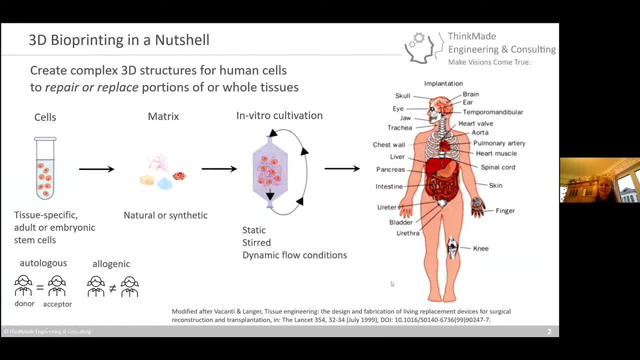 portions or even whole tissues, And that is basically the dream that you have something which is damaged and you can just change that. So, as we heard today, we are not quite yet there. So there are many, many approaches, many, many very interesting technologies. 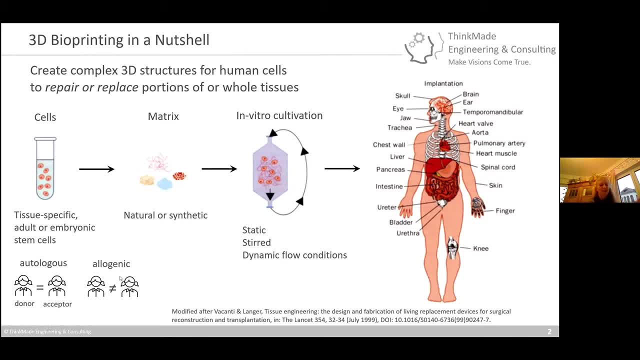 and I tried in the preparation to dive into that issue again. So it starts with cells and matrices, in vitro cultivation and so on, with many different things. you can do with autologous or allergenic cells. So autologous seems to me as a non-biological 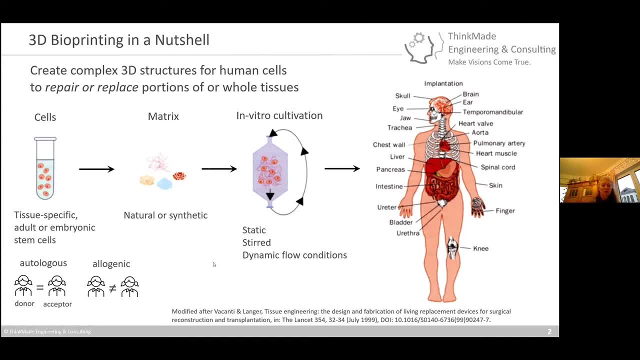 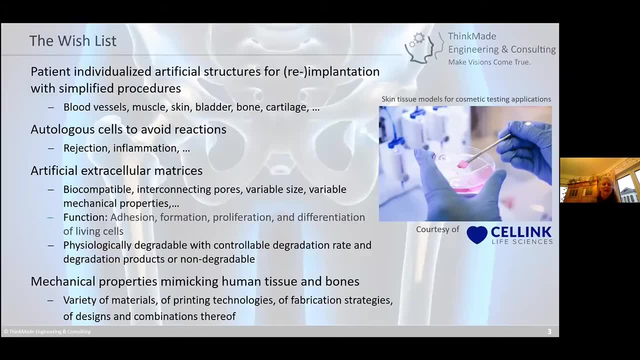 biologist much more likely, because you actually can avoid repulsion and inflammation, reactions and so on, And there is quite a huge wish list of what people would like to see when they talk about this type of thing. So what the idea is? you have a patient, individualized, artificial. 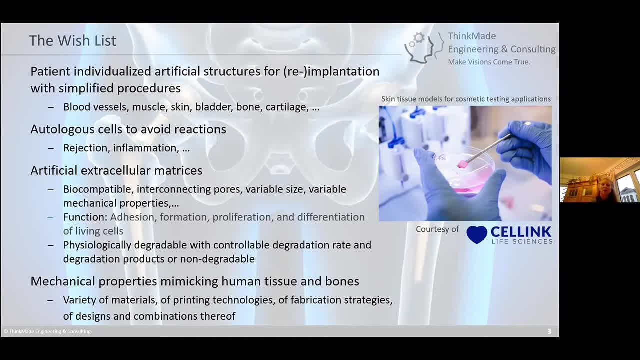 structures which can be used for implantation or re-implantation. So what we heard today, so the autologous cell, seems to be a very good start there And we were very much looking with a biologist into the area of providing artificial extracellular matrices. 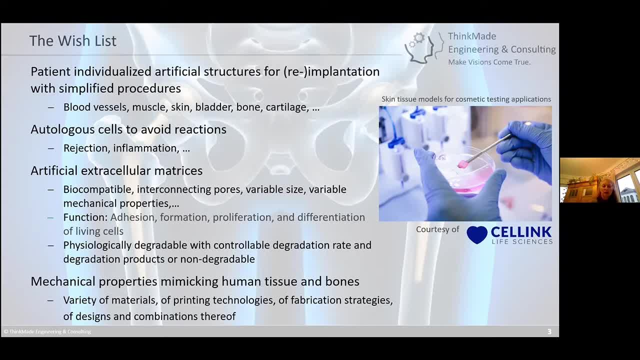 which should be biocompatible with a cell. So we have a very good start there And we have a huge variety of interconnecting pores and variable size and variable mechanical properties to mimic the tissues and to be very, very good adherence for cells. So adhesion and formation. 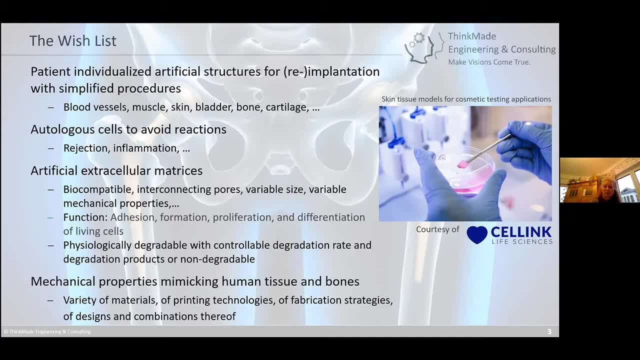 proliferation and differentiation of the living cells was one of our scopes. And also, was it possible, would it be possible, to have a physiologically degradable material Which have controllable degradation rate and degradation products, or non degradable materials which actually can be used in the tissue engineering part? So for the mechanical 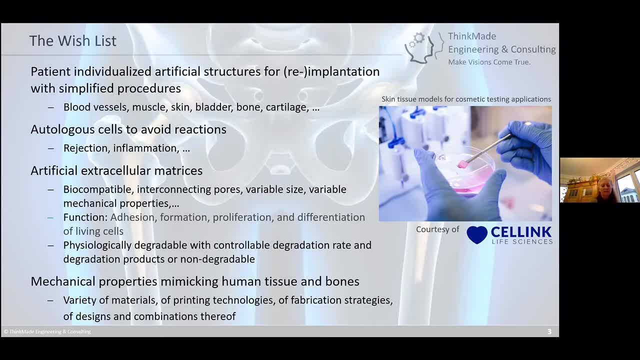 properties. so we heard all that already. It's a variety of materials necessary, actually, in order to fulfill all these different things here. So where's my here? there it is, Umm you. you see my mouse here. Can you see my mouse? 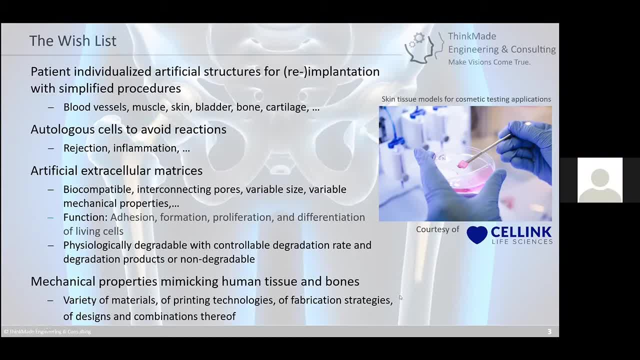 Can you hear me? Yes, yes, Ah, great, Perfect. So, um, printing technology is different. printing technology is different fabrication strategies. So for- once it comes to the three-D printing part, you actually would like to orchestrate, whatever. 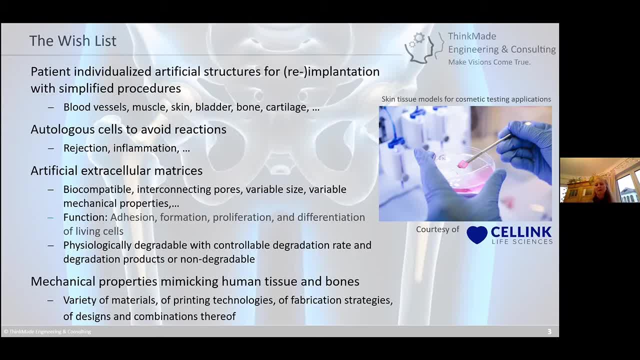 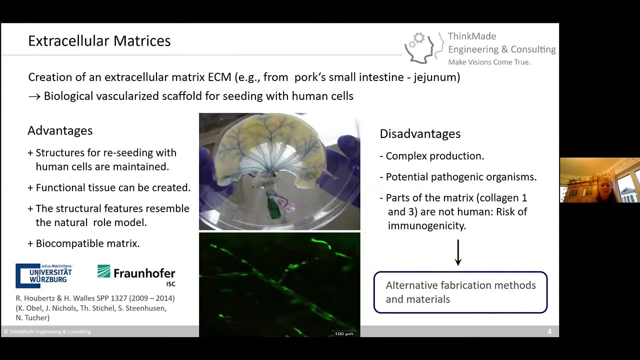 you're doing. you want to get rid of the layer by layer formation and would like to orchestrate your- your- your- functional printing head or whatever, and you would like to have many, many different designs and combinations thereof. So, starting with the extracellular matrices, that was done in cooperation with Heike Wallis. 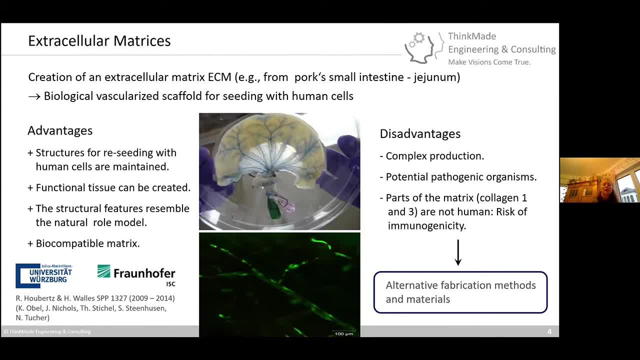 from University of Würzburg, now University of Halle. starting from pork small incestine genome, the dream was to create biological vascularized scaffolds which can be seeded with human cells, and there are many advantages in creating such a structure, which you actually 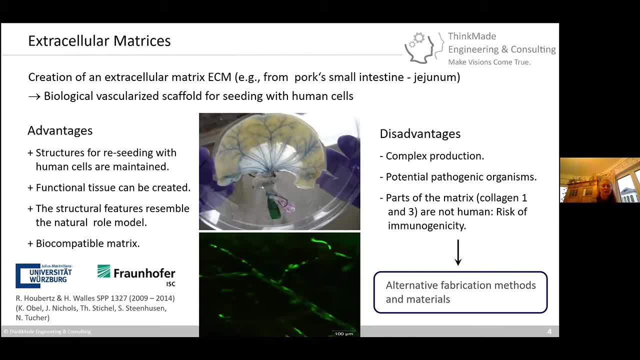 see, you can create functional tissues and you have structural features which resemble the natural role model: biocompatible matrix and so on and so on. but there are also many disadvantages, like a very complex, Very complex production. you have potential, potential pathogenic organisms and part of 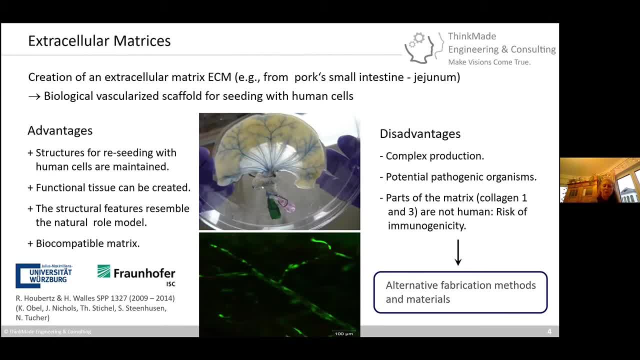 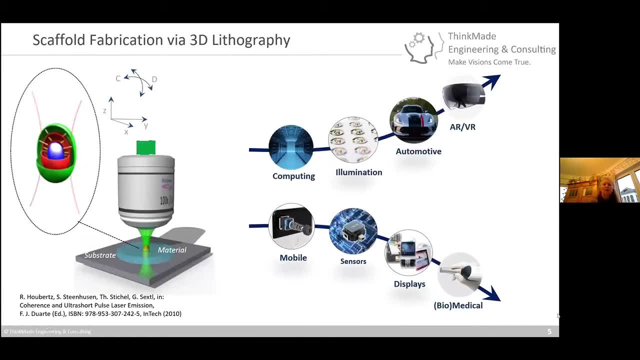 the part of the matrix are not not human. So what we were looking for were alternative, alternative methods, fabrication methods. So what we, what we did and what we started with was scaffold fabrication by a 3D lithography, which is part of the multi photon lithography, and we started very early to expand. 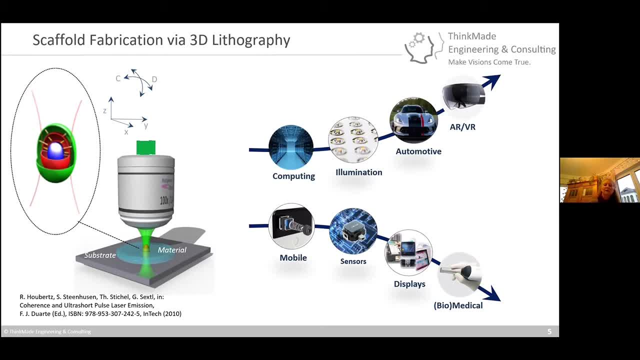 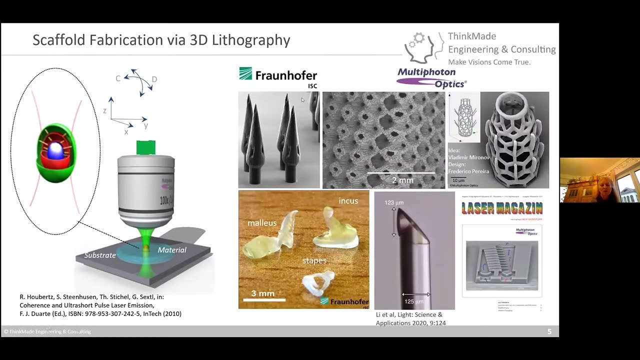 This method from from the pure, let's say, optical and photonics applications into the biology and life science applications, which is very, very important to be- to be combined to other methods, of course, And here are some examples. So, starting with with drug delivery structures and- and this is a little hair cage from Vladimir, 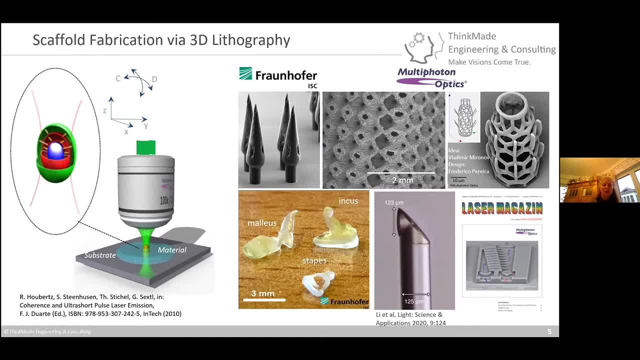 Mironov and Frederick Pereira, who designed that for hair: re implantation of hair follicles, scaffold matrices, complete ear bones. That is an example from from University of Stuttgart, which I actually very like very much, as well as microfluidic cells. 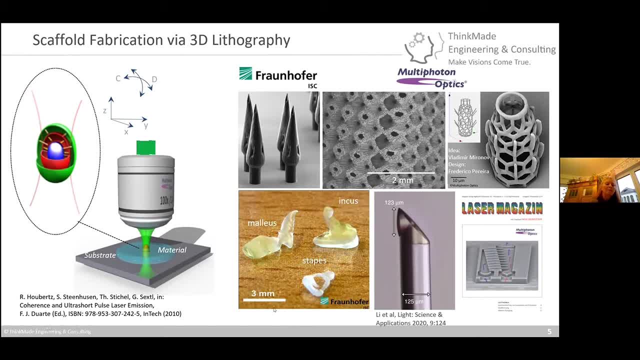 So there is a whole zoo of of what you can basically do, and the feature is was already explained in the in the printing conference. So we use laser light to to create these structures and the reactions are just initiated in a very small focal volume, And it's now a challenge to expand this small focal volume to a to a very large scale. 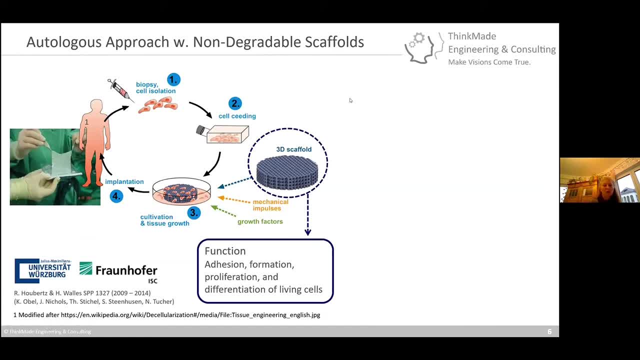 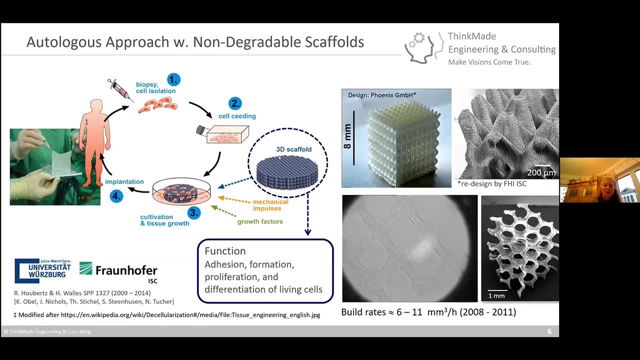 So, starting with the autologous approach with non degradable scaffolds, So you extract the cells and the cell seeding and then you create your scaffolds and put the scaffolds into a cultivation and tissue growth with mechanical and other growth factors. And here are some examples from from 2008 to 2011, where this already was world record. 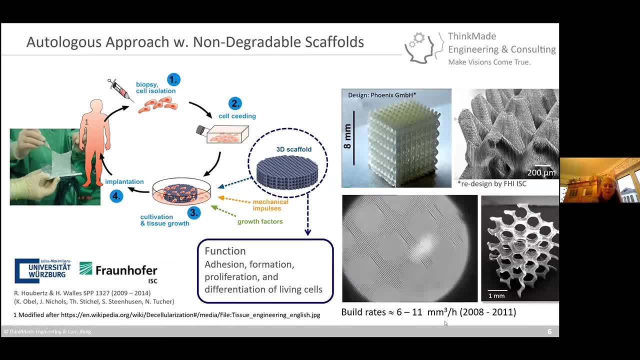 in size and the building rates were quite, quite low at that time. But indeed we could create any, any, any kind of of different, different tissues, different scaffolds here which could be seeded with, with living cells, And the idea is to to re implant that, either by keeping the structure or by having a biodegradable. 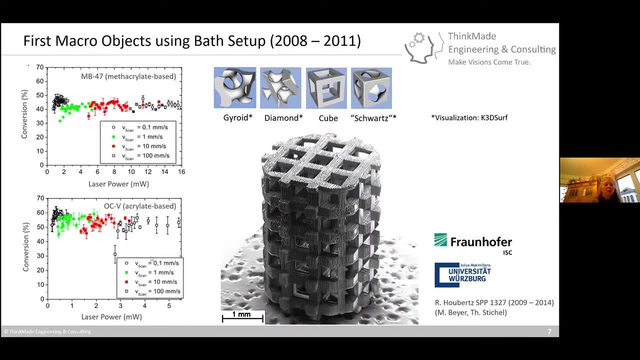 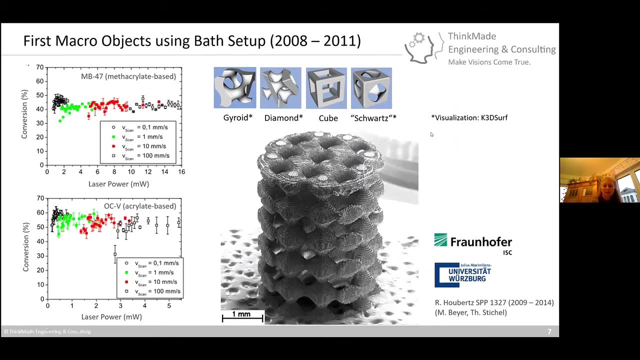 material. So what we did then is when, once you talk about different, different mechanics, you need structures which have different mechanics from different materials. So we started with all these types of diary, diamond, cube and Schwarz structures and created scaffolds from that to investigate whether this is possible. 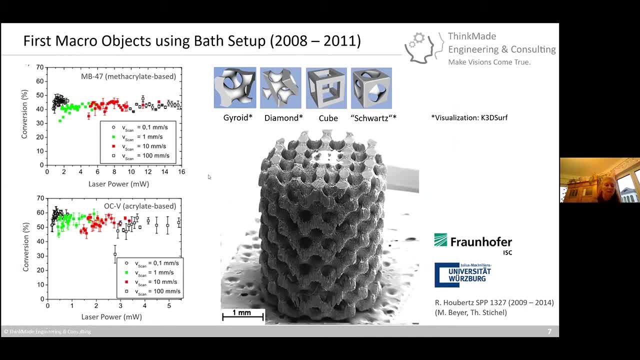 And that was done in the framework of a PhD thesis of Thomas Stichel, And this is a material which was created by Matthias Bayer And we investigate it by by micro Raman spectroscopy, whether this material can be cross linked or whether we can speed up the process. 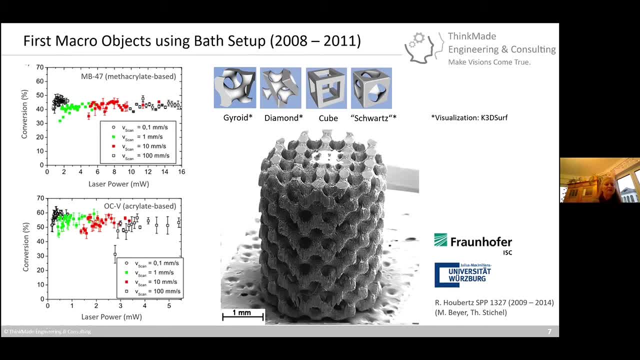 So here is the scan rate of of our laser beam And you see, for any of these speeds you can actually get the same level of of cross linking initiated by the light. So this is a method relate based system. You also can use a method, an accolade based system. 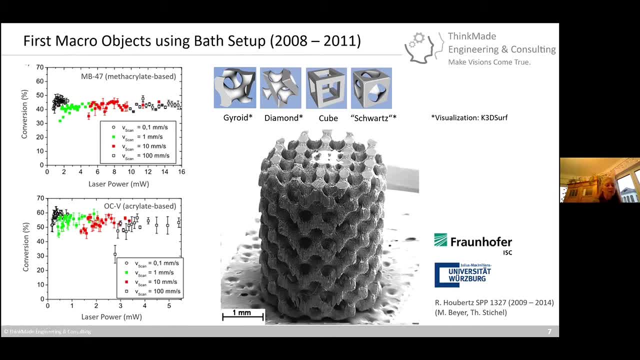 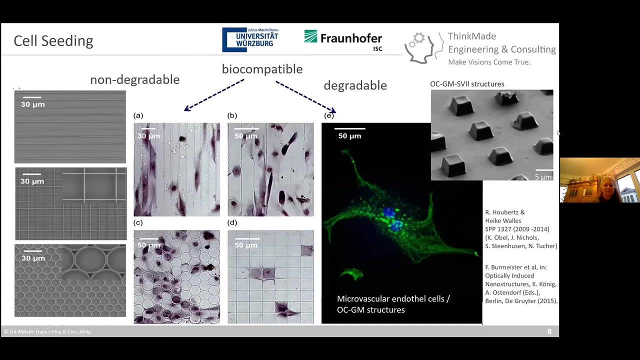 You see, the level of cross-linking of conversion is higher and you also see that the average laser power you need for this material is much lower than for this material to create a solid structure. So we investigated how these structures influence the adhesion and proliferation and differentiation of cells. 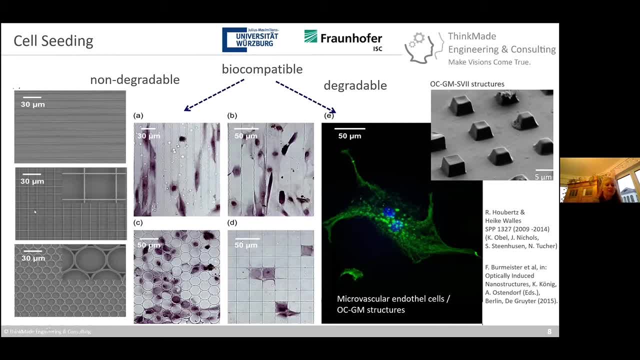 So here you see different examples like longitudinal structures, square structures, circular structures, And what you see from the images here is that the longitudinal structures and the round-shaped structures seem to be alike by the cells, whereas the rectangular structures are not that populated. 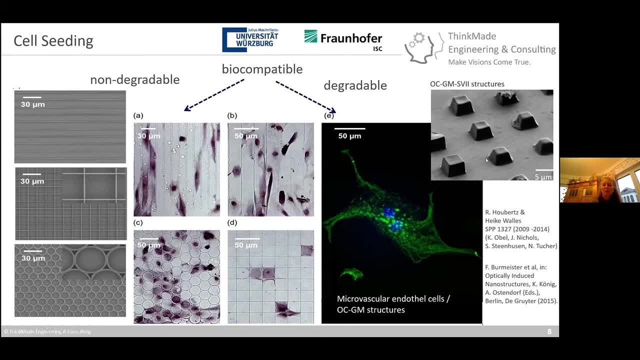 And on this side you see an example of a degradable material, which was done in the framework of a PhD thesis of Kerstin Orbel, where we created the first degradable material. And here you see a microvascular endothelial cells on this material, where you also see cell separation here. 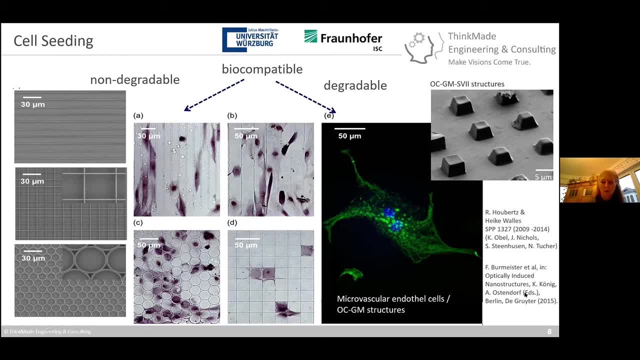 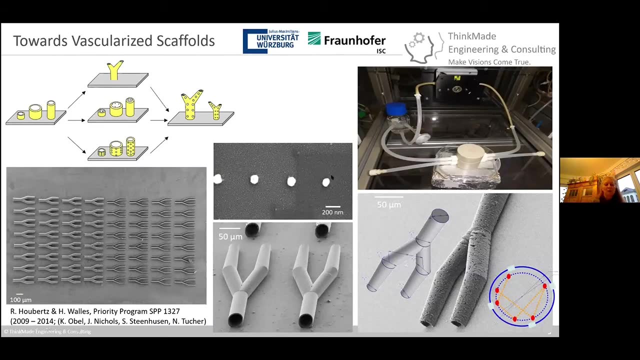 So that was quite interesting. We started very frustrated with our degradation because all our cells always died in the beginning and that was related to the production of alcohol in the cells. They just got drunk and died by the alcohol And once we found that out, that was quite good. 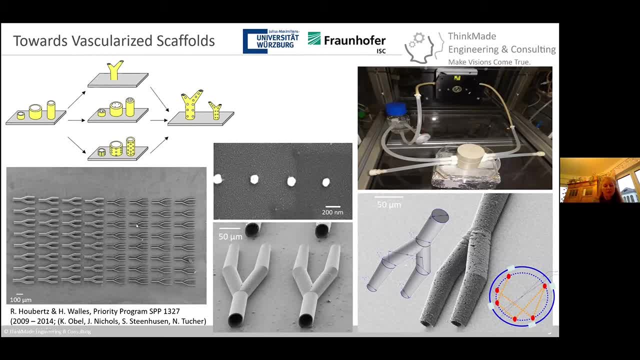 Then we looked into What kind of structures can we do? Can we do tubular structures? And you see that here. So you see a study on a parameter study on tubes which you can then use, which you can then prepare with pores and with little knobs in order to provide links to the cells. 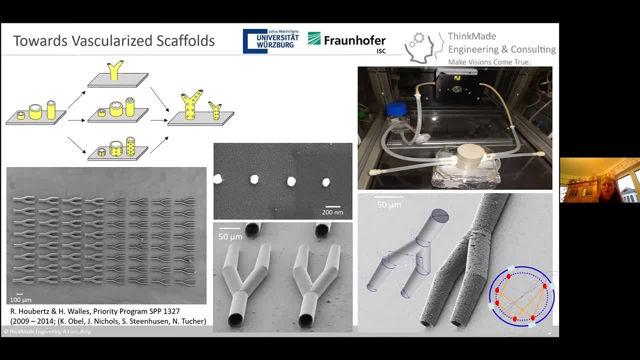 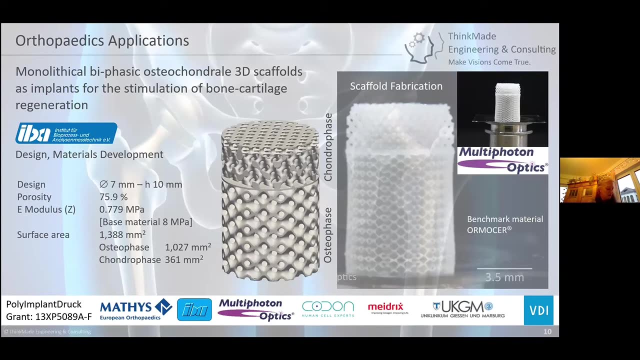 And here is the reactor which was used by Heike Wallis in order to put these materials into this reactor And then use the cells to grow on these type of structures. Orthopedics applications is another application we're looking into, And that was done in my former company, Multifilter and Optics, together with many, many project partners. 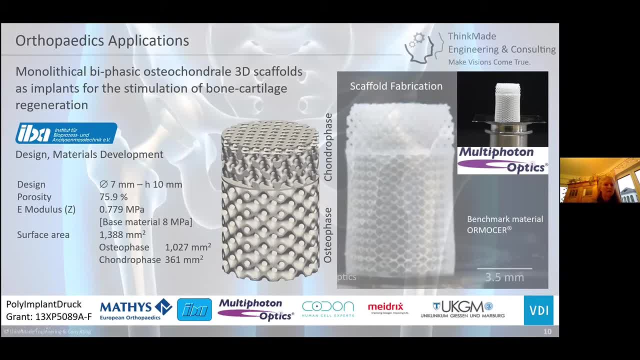 And one partner we work very closely with is the IBA Institute for Bioprocess and Analyse Technique, So they are responsible for the design, So they are responsible for the design And the materials development. So what they came up with is like osteophase and chronophase materials. 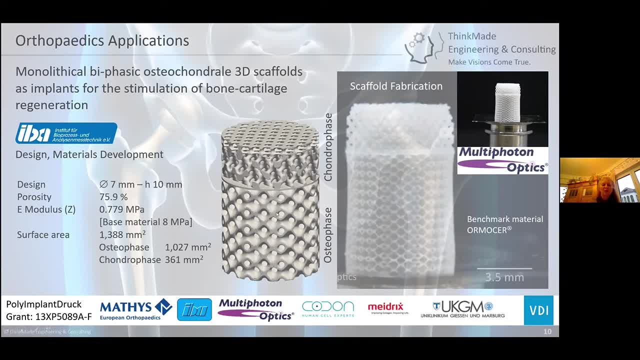 And what we wanted to achieve is a biphasic scaffold, And you remember the studies I've shown on the different structures you can create. So here is the scaffold made from almost a material as a benchmark material, So the total structure is like 7 millimeters in diameter and about a centimeter in height. 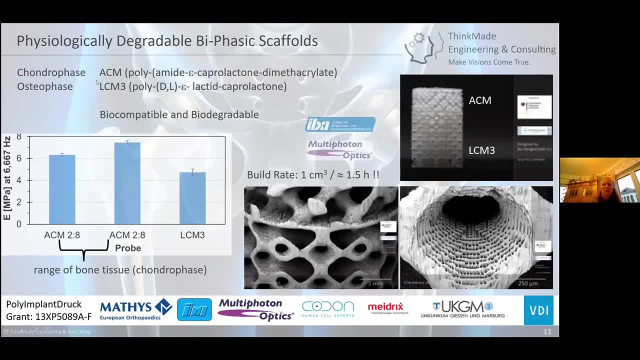 And with that we use the materials ACM and LCM3, which is polyamide Epsilon Caprolectone demethacrylate and polyDL Epsilon Lactide Caprolectone for the other phase, And investigated also the mechanical properties of this material. 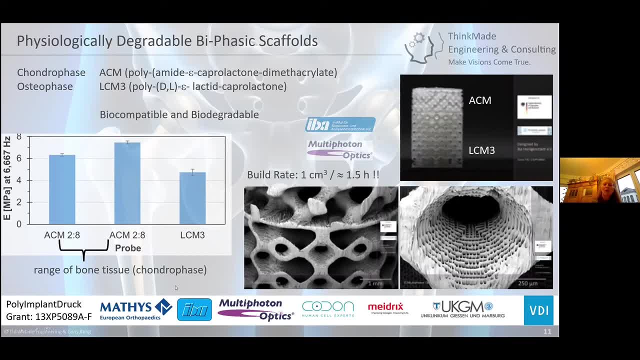 And here you see a very, very nice example of a of a biphasic scaffold. and remember the build rate I've shown you from 2014. here the build rate is about a square centimeter in- sorry, a cubic centimeter- in about 1.5 hours. so it's. 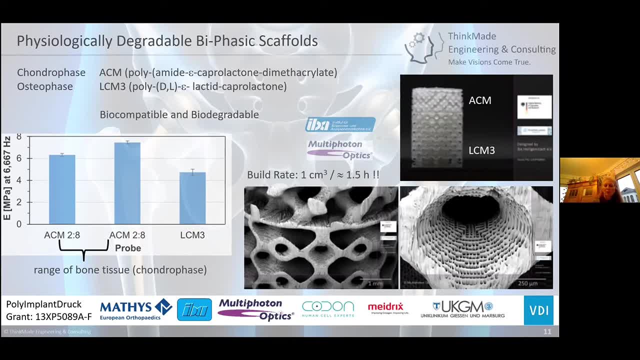 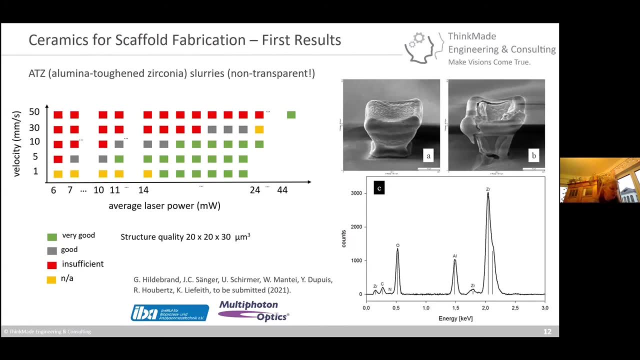 100 times faster. that was done with new equipment we developed throughout this project. We also looked into ceramics for scaffold fabrication, so this is a little bit challenging because these ceramics are slurries and they are not transparent, so the idea is to focus your beam into a transparent bath. but the good news is we even found parameters for the ceramics. 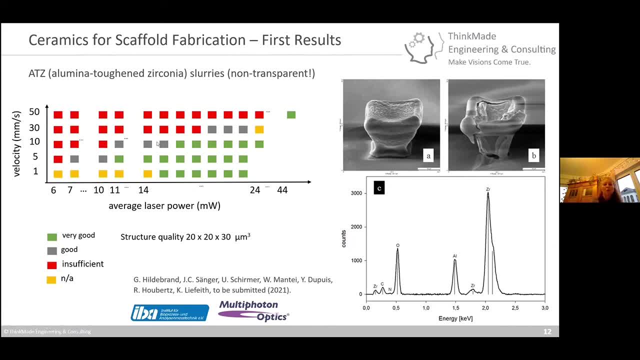 and process parameters and process windows to create ceramic polymer structures, which is shown here and after debending, you see the structure here. it's not the perfect, but it's obvious that we're working on it. We're able to do that and we're now looking into creation of ceramic scaffolds. of course, 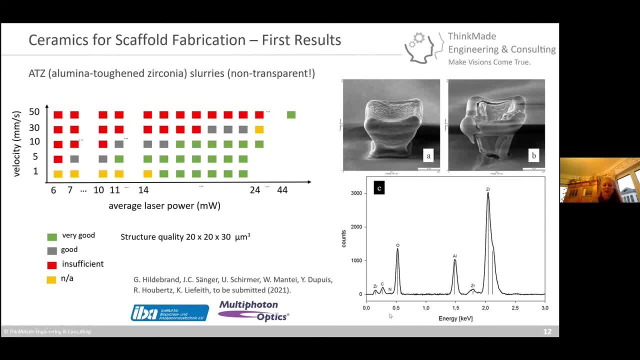 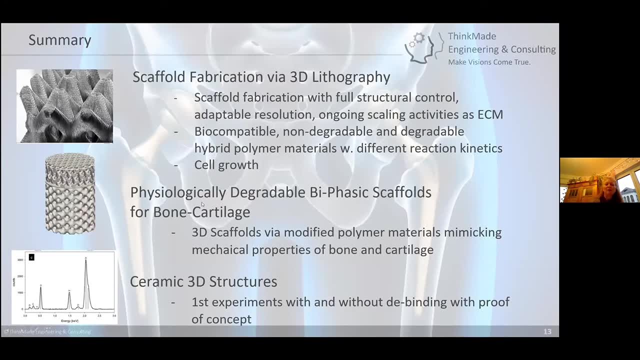 and here you see an x-ray image of the ceramic phase after debending. so I hope I could show you some examples on the scaffold fabrication, where we have full structure control, adaptable resolution and there are ongoing scaling activities for the extracellular matrices. the materials are biocompatible, non-degradable or degradable hyperpolymer materials with different 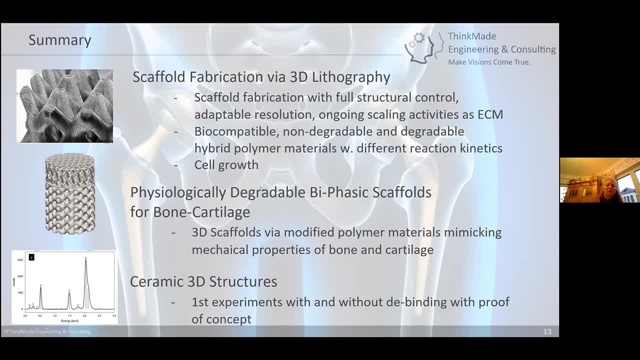 reaction kinetics from the material class of the homocere of the renacer, which is a new material class invented about, let's say, 20 years ago. cell growth is ongoing. I've shown the examples on physiologically degradable biphasic scaffolds for bone cartilage and the cell growth is ongoing. 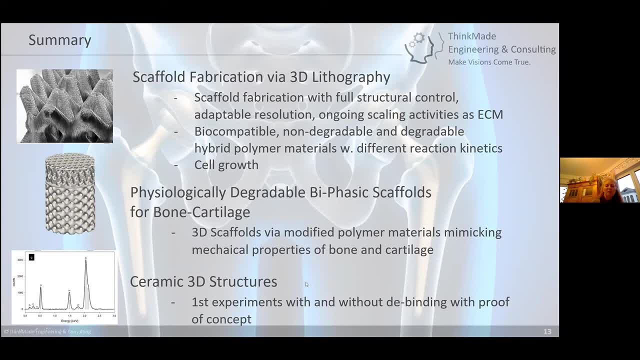 applications and the mechanical properties are mimicked by the, by the structure and by the materials and first cell cultures and showed that they are compatible and biocompatible, as well as first examples of ceramic 3d structures as a first proof of concept. so this works of 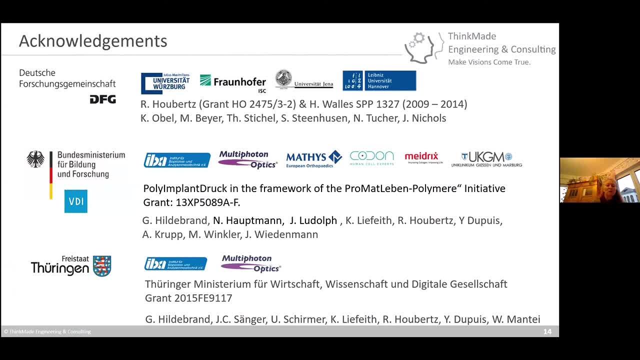 course was were not done by myself, so I part of the work was initiated by myself. so that was the German science foundation project with PhD students you see here and the the diploma student and people from from Heike Wallis group as well, and also the vmbf funded project poly implant hook.